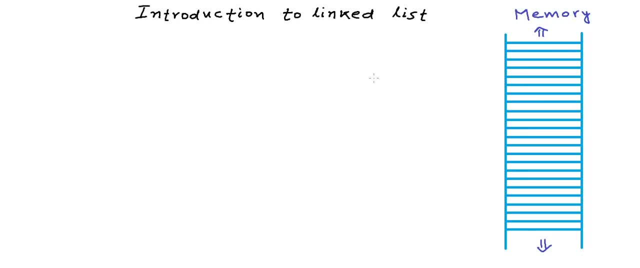 To help you understand this, let us say this is computer's memory and each partition here is one byte of memory. Now, as we know, each byte of memory has an address. We are showing only a section of the memory. That's why it is extending towards the bottom and the top. Let's say the address increases from bottom to top. So if this byte is address 200, the next byte would be address 201, and next byte would be address 202, and so on. 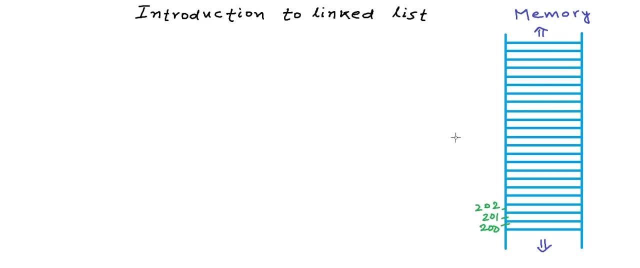 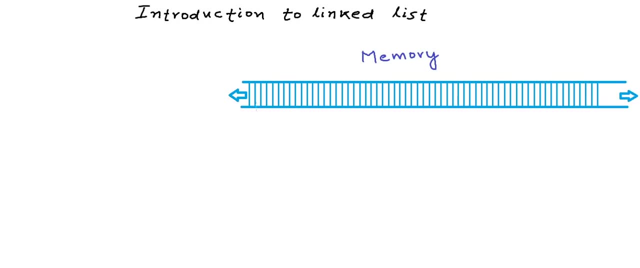 What I want to do is I want to draw this memory from left to right horizontally instead of drawing it from bottom to top like this. This looks better. Let's say this byte here is address 200, and as we go towards the right the address increases. So this is like 201 and we go on like 202, 203 and so on. It doesn't really matter whether we show memory from bottom to top or left to right. These are just logical ways to look at the memory. 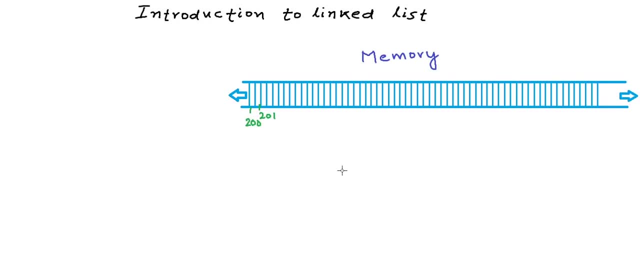 So, coming back to our story, memory is a crucial resource and all the applications keep asking for it. So Mr Computer has given this job of managing the memory to one of his components, to one of his guys, who he calls the memory manager. Now, this guy keeps track of what part of the memory is free and what part of the memory is allocated, and anyone who needs memory to store something needs to talk to this guy. 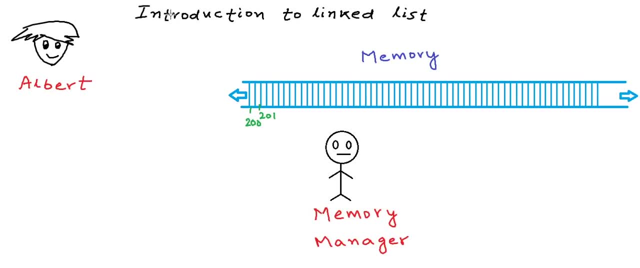 And he is building an application. He needs to store some data in the memory, So he needs to talk to the memory manager. He can talk to the memory manager in a high level language like C. Let us say that he is using C to talk to the memory manager. First, he wants to store an integer in the memory, So he communicates this to memory manager by declaring an integer variable, something like this: The memory manager sees this declaration and he says that: okay. 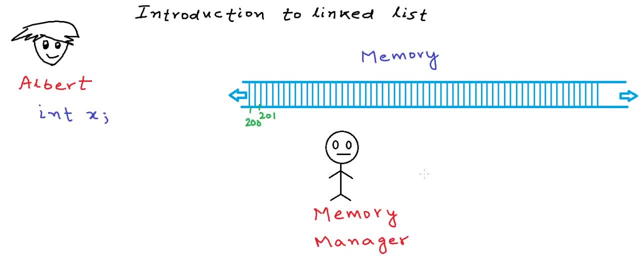 if you want an integer variable, you need to store an integer variable. so I need to give you four bytes of memory, because integer variable is stored in four bytes in a typical architecture. Let us say: in this architecture it is stored in four bytes, So the memory manager looks for four bytes of free space in the memory and assigns it or allocates it for variable x. 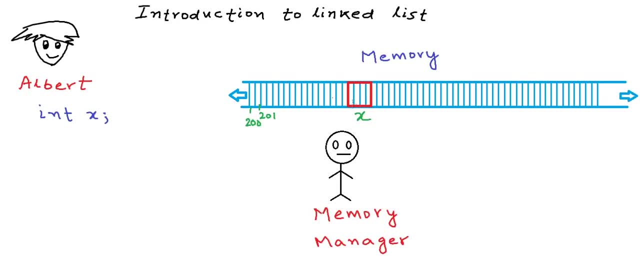 Address of a block of memory is the address of the first byte in the memory. So let us say this first byte of memory memory here is at address 217. so variable X is at address 217.. So memory manager kind of communicates it back to Albert that hey, I have assigned address 217 for your. 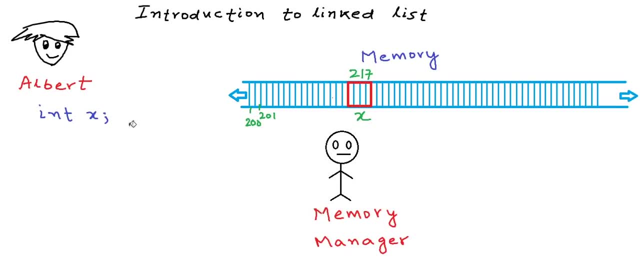 variable X. You can store whatever you want there and Albert can fill in any data into this variable. Now Albert needs to store a list of integers, a list of numbers, and he thinks that the maximum number of integers in this list will be 4.. So he asks: 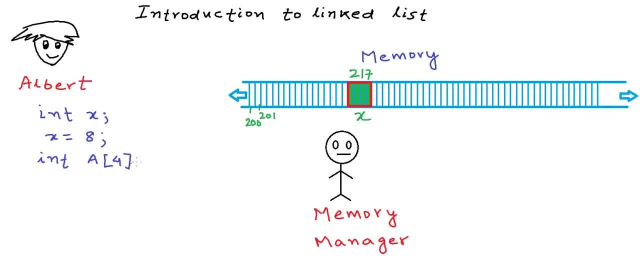 the memory manager for an integer array of size 4 named A. Now, array is always stored in memory as one contiguous block of memory. So memory manager is like: okay, I need to look for a block of memory of 16 bytes for this variable, this array A. 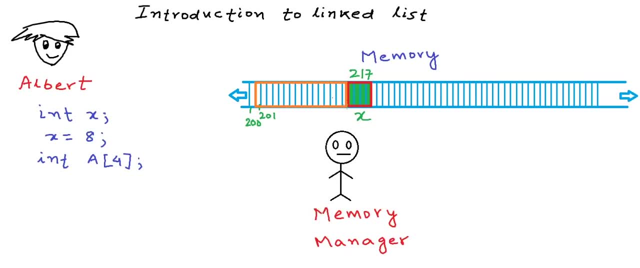 So the memory manager allocates this block starting address 201 and ending address 216 for this variable A, which is an array of four integers. Because array is stored as one contiguous block of memory and memory manager conveys the starting address of this block whenever Albert tries to access any of the elements in the 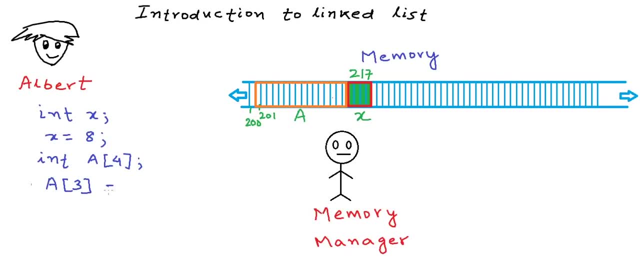 array let's say he tries to access. let's say he tries to write some value at the fourth element in the array which he accesses, as A Albert's application knows where to write this particular value because it knows the base address, the starting address of the block A. 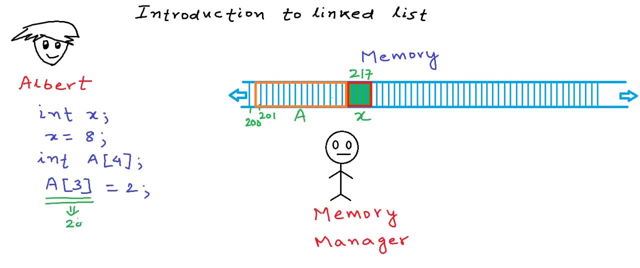 the array A and from base address, using the index, which is 3, here it calculates the address of A3. So it knows that A3 is at address 213.. So to access any of the elements in the array, the application takes constant time and this: 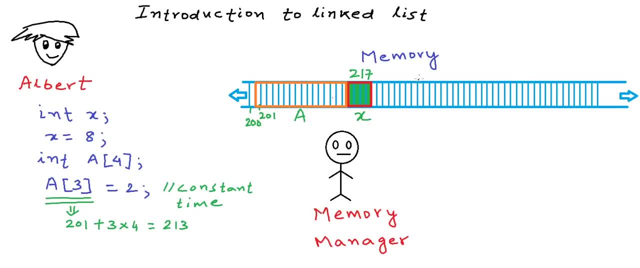 is one awesome thing about arrays: that, irrespective of the size of the arrays, the application and application can access any of the elements in the array in constant time. Now let's say Albert uses this array of four integers to store his list, So I'll fill in some values here at these positions. let's say: 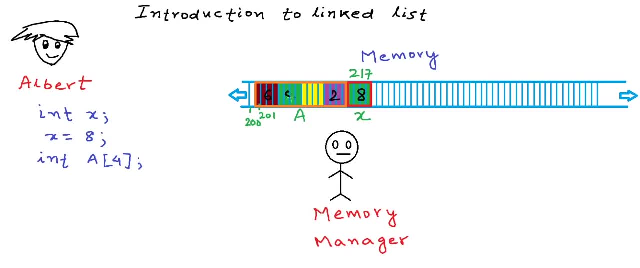 this is 8,, this is 2,, this is 6,, this is 5,, this is 4.. Now Albert at some point feels that, okay, I need to have one more element in this list. Now he has declared an array of size 4 and he wants to add: 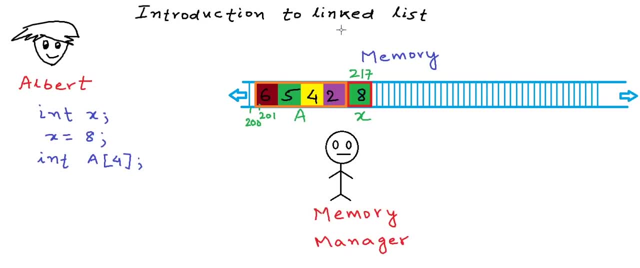 a fifth element in the array. So he asks the memory manager that, hey, I want to extend my array A. Is it possible to do so? I want to extend the same block and the memory manager is like: when I allocate memory for an array, I do not expect that you will ask for an extension. so 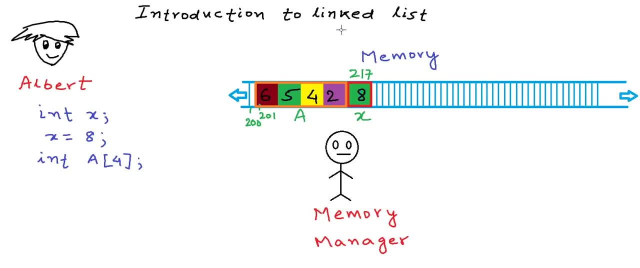 I use whatever memory is available adjacent to that block for other variables. In some cases I may extend the same block, but in this case I have an element and a variable X next to your block, so I cannot give you an extension. So, Albert is like what all options do I have? 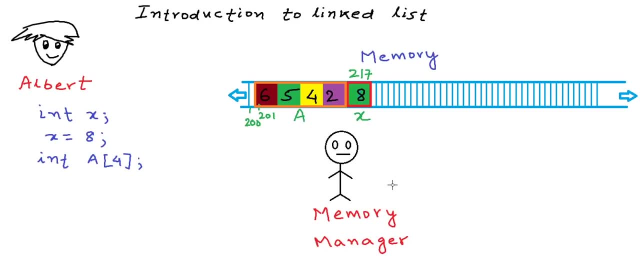 Memory manager is like: you can tell me the new size and I can recreate a new block at some new address and we will have to copy all the elements from the previous block to the new block. So Albert says that okay, let's do it. but the memory manager is like: 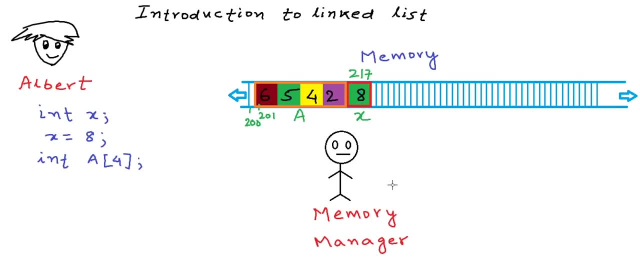 you still need to give me the size of the new block. Albert thinks that this time he'll give a really large size for the new array or the new block, so that it does not fill up This new block. starting address 2 to 4. 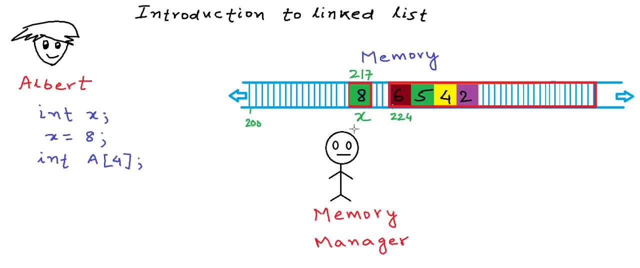 is allocated, Albert asks memory manager to free the previous block, and this is some cost. he has to copy all the elements, all the numbers from the previous block into the new block, and now he can add one more element to this list and he has kept his array large. 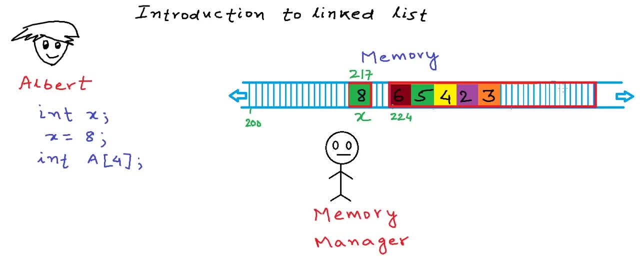 this time, just in case he needs more numbers in the list. So the only option that Albert had was to create A as an entirely new block, as an entirely new array. and Albert is still feeling bad because if the list is too small, he is not using some part of the array, and so memory is getting wasted. 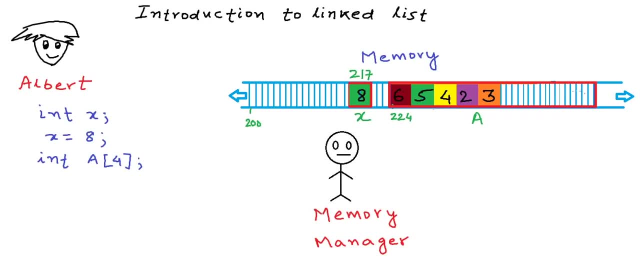 and if the list again grows too much, he will again have to create a new array, a new block, and he will again have to copy all the elements from the previous block into the new block. Albert is desperately seeking a solution to this problem, and the solution to this problem is a data structure. 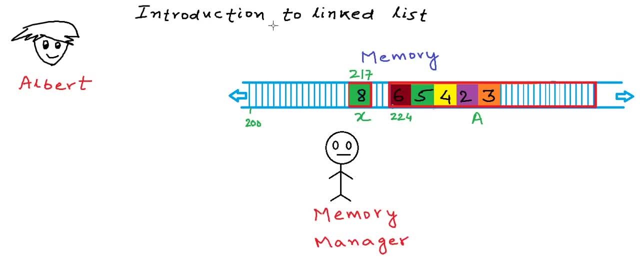 named linked list. So let us now try to understand linked list data structure and see how it solves Albert's problem. What Albert can do is that, instead of asking the memory manager for an array, which will be one large contiguous block of memory, he can ask memory for one unit of data at a time. 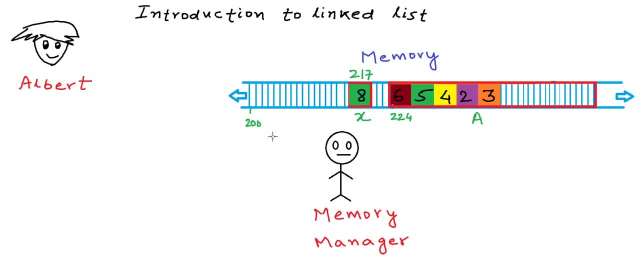 for one element at a time in a separate request. I'm cleaning up the memory here Once again. let's say Albert wants to store this list of four integers in the memory. What if he requests memory for one integer at a time? So first he pings memory manager for some memory to store number six. 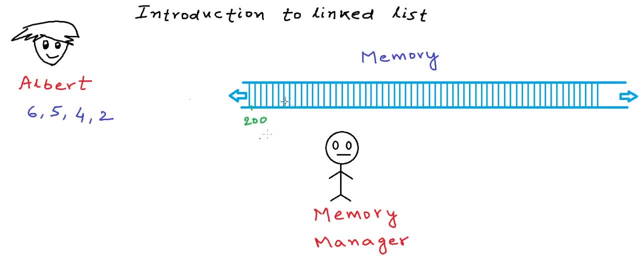 Memory manager will be like: okay, you need space to store an integer, so you get this block of four bytes at address 204.. So Albert can store number six here. Now Albert makes another request, a separate request, for number five. Let's say he gets this. 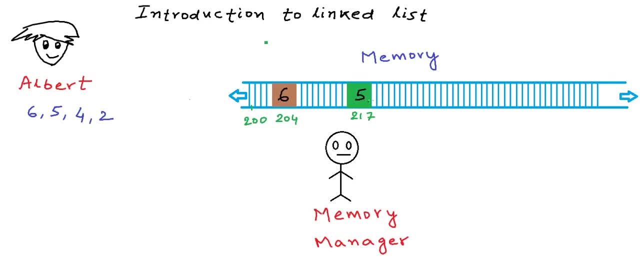 block starting address 217 for number five Because he makes a separate request. he may or may not get memory adjacent to number six. Higher probability is that he will not get an adjacent memory location. So similarly, Albert makes separate requests for number four and two. So let's say he gets. 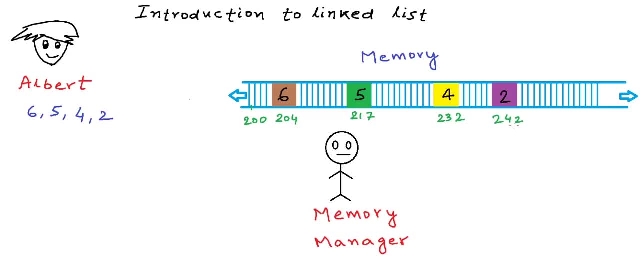 these two blocks at address 232 and 242, respectively for numbers 4 and 2.. So, as you can see, when Albert makes separate requests for each integer, instead of getting one contiguous block of memory, he gets these disjoint, non-contiguous blocks of memory. 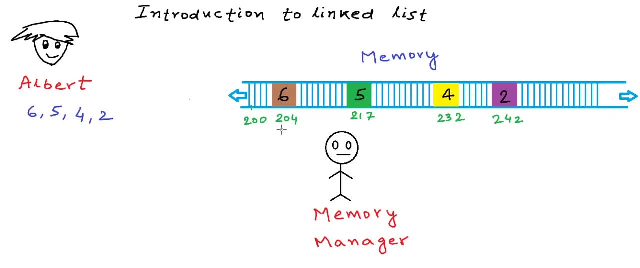 So we need to store some more information here. we need to store the information that this is the first element in this array list And this is the second element in this list. So we need to link these blocks together somehow. With an array it was very simple: we had one contiguous block of memory, So 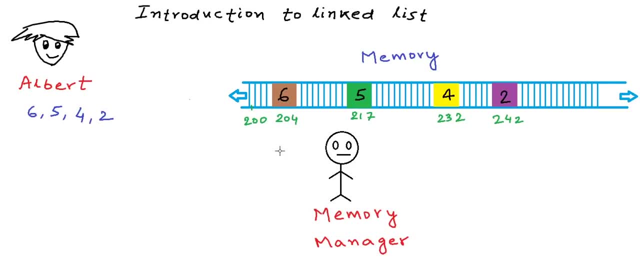 so we knew where a particular element is by calculating its address using the starting address of the block and the position of the element in the array. But here we need to store the information that this is the first block which stores the first element and 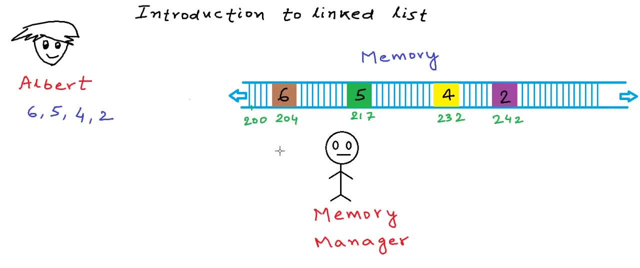 this is the second block, which stores the second element, and so on. To link these blocks together and to store the information that this is the first block in the list and this is the second block in the list, what we can do is that we can store some extra information. 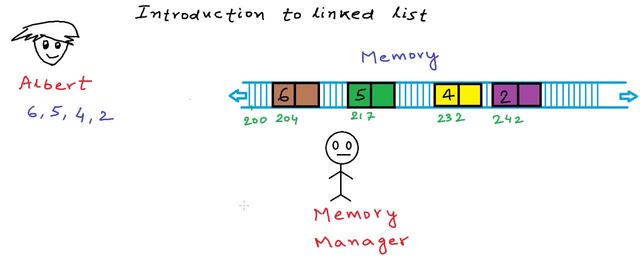 with each block. So what if we can have two parts in each block, something like this: And in one part of the block we store the data or the value, And in the other part of the block we store the address of the next block. In this example, in the first block, the address. 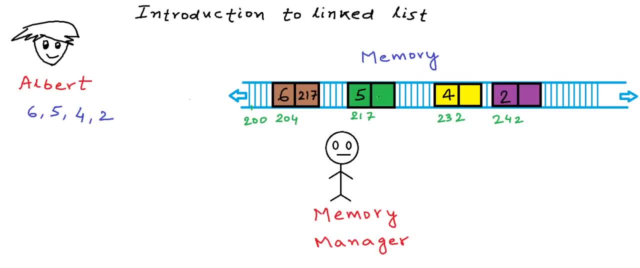 part would be 217.. The address of the next block that stores five And in this next block or the second block, the address part would be 232.. In the block at address 232, we will store the address 242, the address of the next block that stores number two, and the block at 242 is the last. 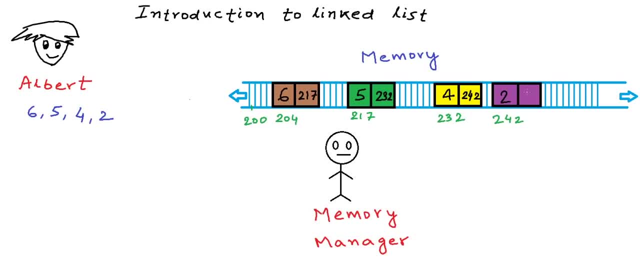 block. there is no next block after this. So in the address part we can have address as zero. zero is invalid address. Similarly, in the episodes we can have address as management number one, building number one, built in building a new event and building an event in the next block after this next. 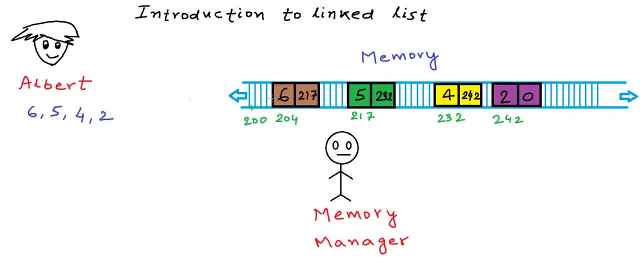 block is valid. So what we have done is that we've saved our first block from the list of buttons. after we have Ravi outwards, we have our center course to connect to the second block, we have the address to the second block and we can start the current development. 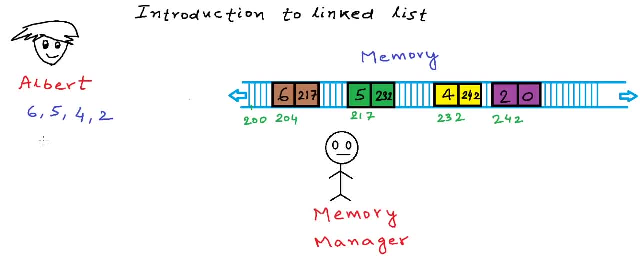 Let me show you what we can do. As you can see開始 a type named node like this. he will have two fields in the node: one to store the data- this field will be an integer- and one more field to store the address of the next node in the list. so Albert will ask a node, Albert will ask memory for a. 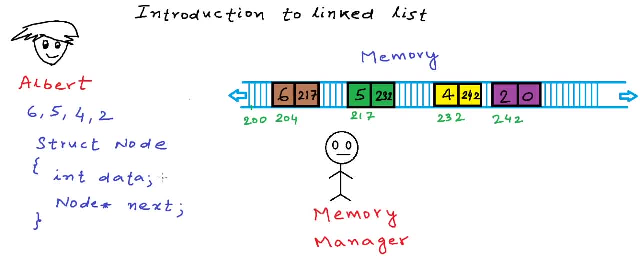 node from the memory manager and the memory manager will be like: okay, you need a node that needs 4 bytes for an integer variable and 4 more bytes for the pointer variable. that will store the address pointer variable. also, in a typical architecture is stored in 4 bytes. so now memory manager gives us a 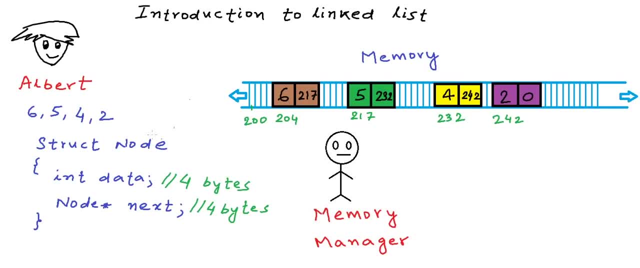 block of 8 bytes and we call this block a node. now notice that the second field in the node structure is node star, which means pointer to node. so this field will only store an address of the next node in the list. so if we store the list like this in the memory as these: 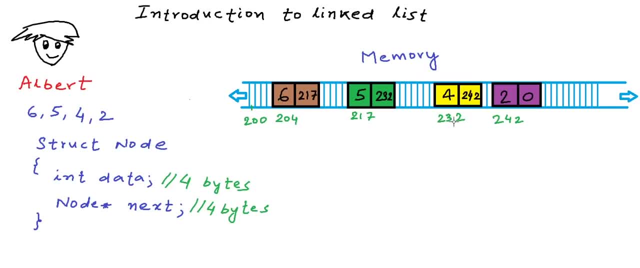 non-contiguous nodes connected to each other. now, then, this is a linked list data structure. logical view of the linked list data structure will be something like this: data is stored in these nodes and each node store the data as well as the link to the next node, so each node kind of points to the next node, the. 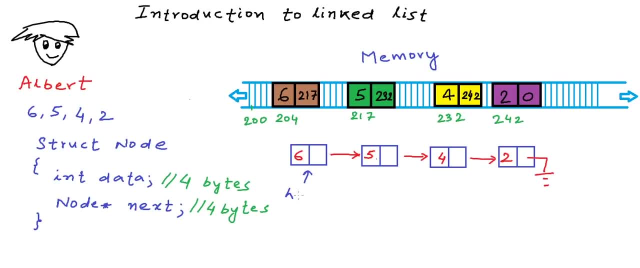 first node is also called the head node, and the only information about the list that we keep all the time is address of the head node or address of the first node. so address of the head node kind of gives us access to the complete list. the address in the last node is null or zero, which means that 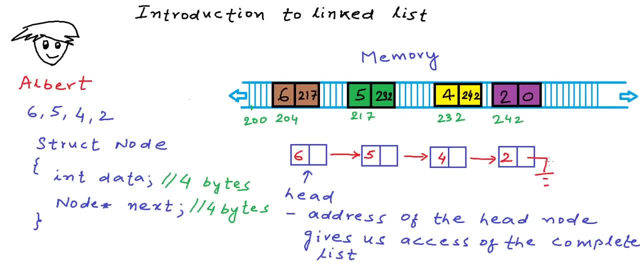 the last node does not point to any other node. now, if we want to traverse the linked list, the only way to do it is we start at the head and we go to the first guy, and then we ask the first guy the address of the next guy. 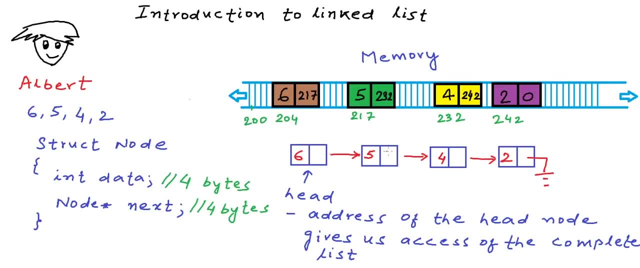 address of the next node. and then we go to the next node and ask the address of the next node and this is the only way to access the elements in the linked list. if we want to insert a node in the linked list, let's say we want to add. 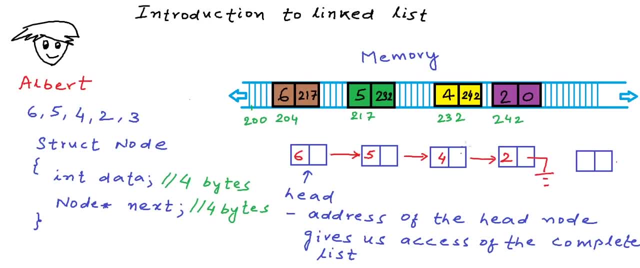 number 3 at the end of the linked list. then all we need to do is first create a node in the linked list- sorry, first create a node independently and separately. it will get some memory location. so we created this node with value 3. now all we need to do is create a node in the linked list and then we. 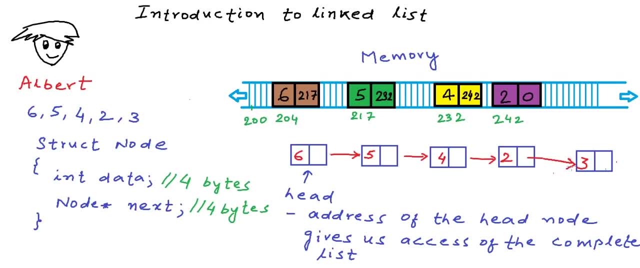 need to do is fill the address properly, adjust these links properly so the address of this particular node will be filled in this node with value 2 and this node- the address part- can be null. so it is the last node. it does not point to any other node. let's also show this, these nodes in the memory here. so I've 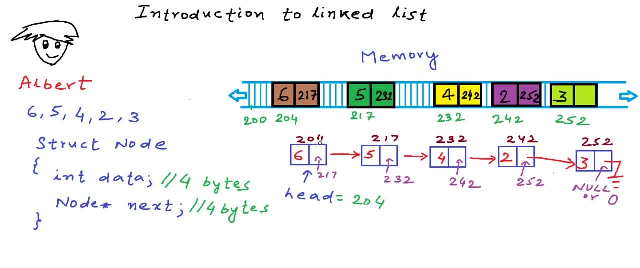 written the address of each node in brown at top of these nodes and I've also filled in this address field of each node. let's say, the node for value 3 gets address 252. so this is how things will be in the memory and this is how the logical view will be the linked list. 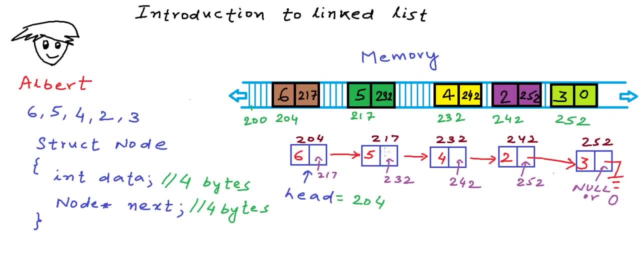 is always identified by the address of the first node and, unlike arrays, we cannot access any of the elements in constant time. in the case of arrays, using the starting address of the block of memory and using the position of the element in the list, we could calculate the address of the element, but in this 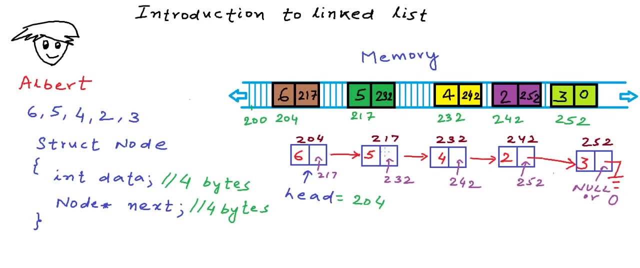 case, we have to start at the head and we have to ask this element for next element and then ask the next element: who is your next? it's like playing treasure hunt: you go to the first guy and then you get the address for the second guy, and then you go to the second guy and you get the address for the. 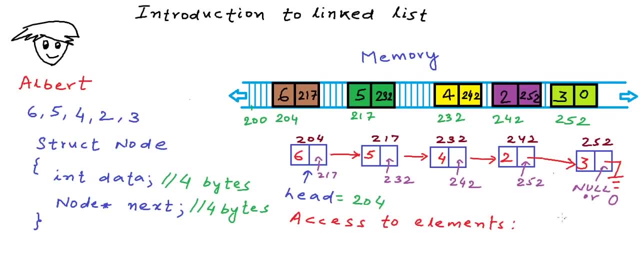 third guy. so the time taken to access elements will be proportional to the size of the list. let's say the size of the list is n. there are n elements in the list. in the worst case, to traverse the last element, you will go through all elements. so time taken to access elements is proportional to n or in. 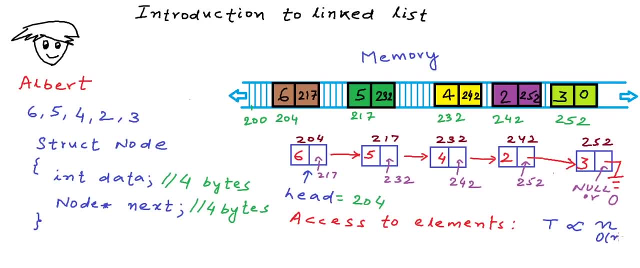 other words, we say that this operation will cost us, or rather the time. complexity of this operation is big. o of n insertion into the list. we can insert anywhere in the list. we first need to create a node and just adjust these links properly, like, say, I want 10 at third position in the list. so all we 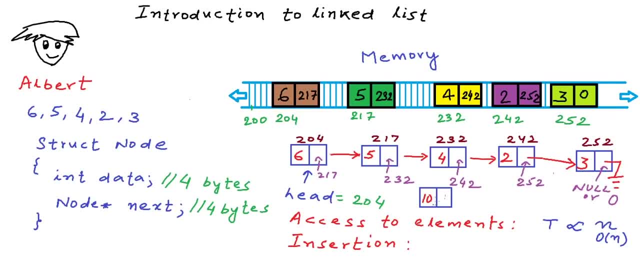 need to do is create a node, store the value 10 in the data part. something like this: Let's say we get the node 10 at address 310. So we will adjust the address field in the second node to point to this node with address. 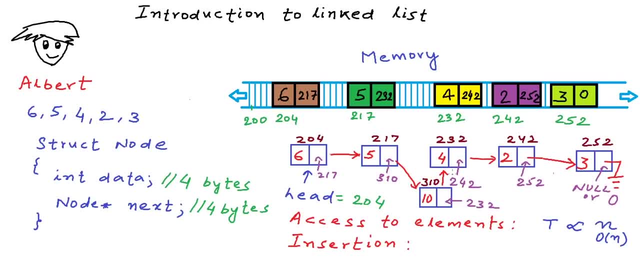 310, and this node will point to the node with value 4.. Now, to insert also, we will have to traverse the list and go to that particular position, and so this will be O again. in terms of time complexity, The only thing is that the insertion will be a simple operation. we will not have to.